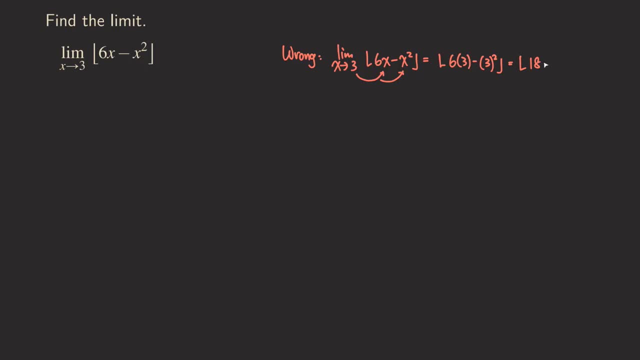 we are going to get what We are going to get: the full function of 18 minus 9, and then we are going to get a whole number right here which is the greatest integral. So if we plug in the integer, when we plug in the 9, which is what? What is that? Just 9, right. 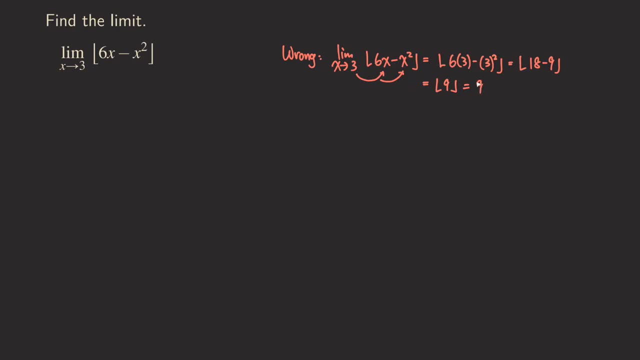 But that is the wrong answer here, So that is bad. Okay, so we don't want this answer here. The reason for why it's bad is that you can actually try to graph this function on decimals and then you will see that the answer is actually not 9.. But then now, how do we do this problem? 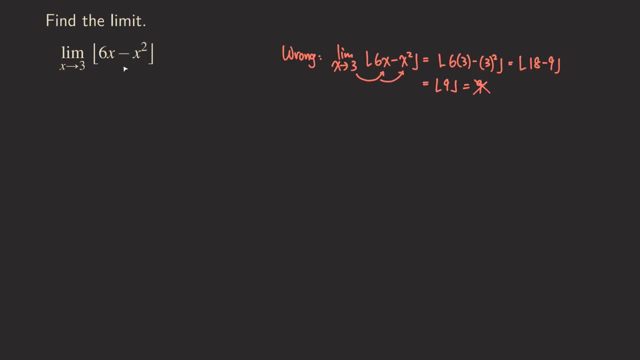 Well, one way to try it is that we can. maybe we can try to factor this function here, the 6x minus x squared, and see what happens. In fact, that also would be approached. that doesn't really work. Now, I'm just going to show. 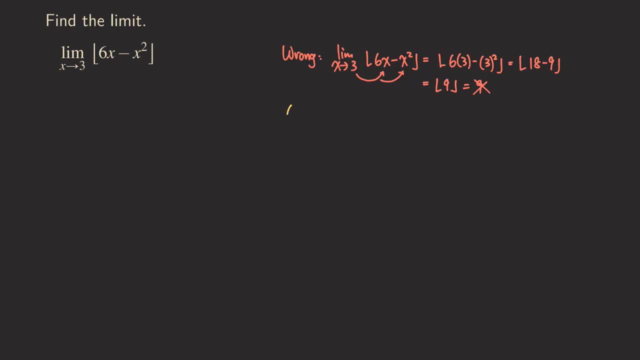 that quickly why that doesn't work. So let's say we factor this 6x minus x, squared right here, and see what happens is that we factor out the x and we are going to get 6 minus x. And so if x is approaching 3, then we can see that this is also approaching 3 and this is approaching 3.. And so 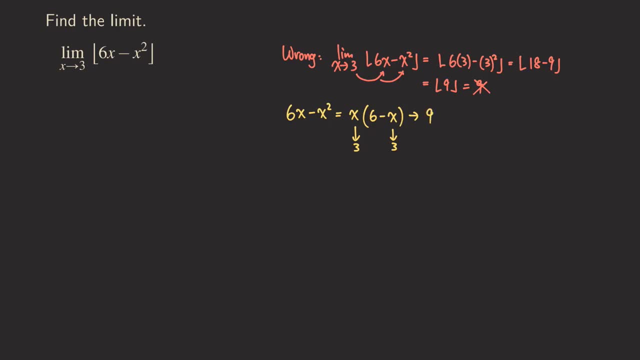 this expression right here- would also be approaching nine, And so you may say soon we'd be considering the one side that limits and see what's going on. Well, we can try that. Let's say if X is approaching three from the left side. 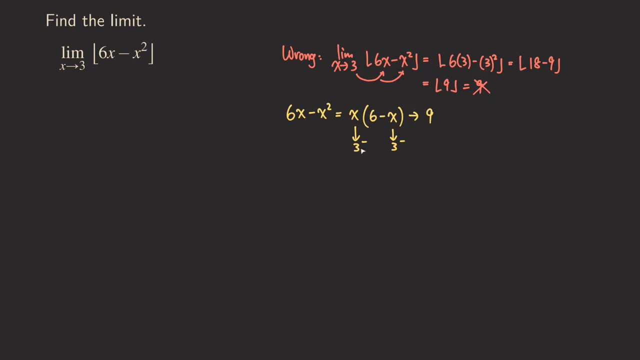 then do you see what's going on here? Well, this X is approaching three from the left side. So it looks like what? looks like 2.9,, 2.99, and then 2.995, and then 2.999, and so on, Right And what. 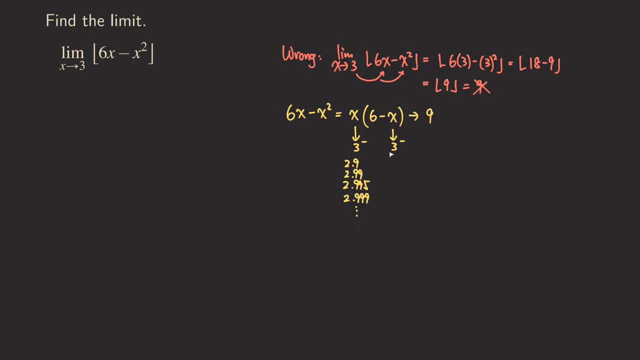 about the other one. This one, when X is approaching three from the left side, then also looks like this right. But when we take the six minus all that, then what happens is that this six minus X would be approaching three from the right side, And so it really looks like 3.01,. 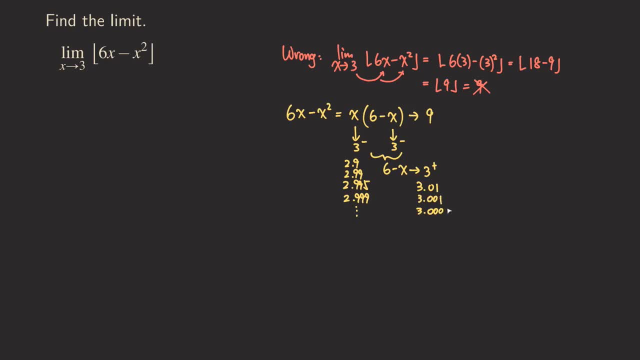 3.001, and then 3.0005 maybe, and then 3.00001 and so on. And you can see that, because when we are doing the multiplication with the X and then also this X minus X, we're actually taking a number that is really close to three on the left side. And then 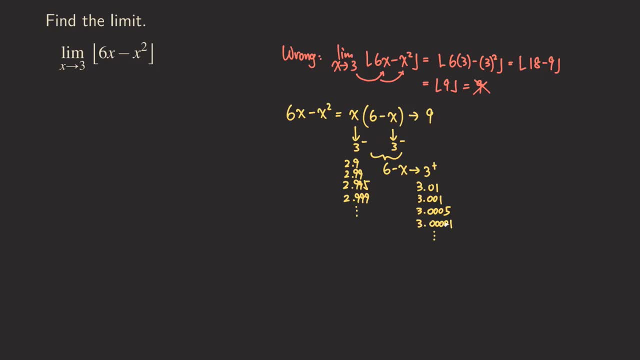 we have a number that is close to three on the right side, And we actually don't know whether that's going to give us something that's less than nine or something that is greater than nine, And both can be possible. So that will not really tell us whether this is actually approaching. 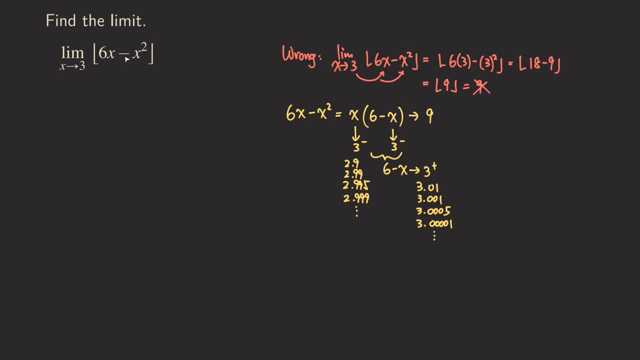 3.01.. Um, nine on the left side or nine on the right side, So that is not going to help. And then you may say: how do we do it then? Now, one way to do it Okay Is that we can actually complete the. 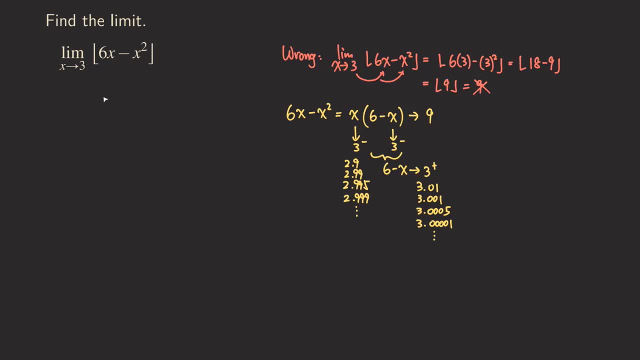 square on this function right here. Then you may say: how do we complete the square? Well, let's take a look. We can first let F of X be six X minus X square, And then we writing this function. then we are going to get a factoring out the um, the latest one from the X square. 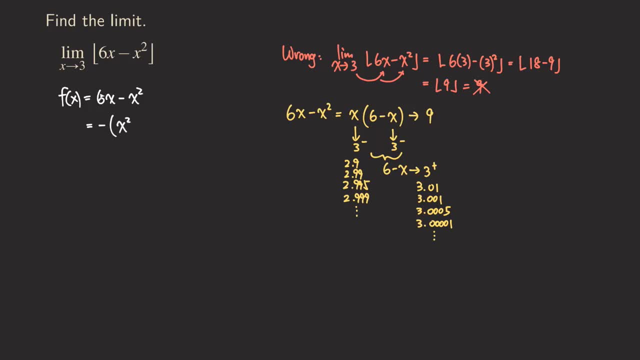 We are going to just get positive X square inside the parentheses, And then, because we factored the latest one, so we are going to change the sign for the six, So we get negative six X. Now we want to complete the square on this expression inside the parentheses. So we are going to get negative and. 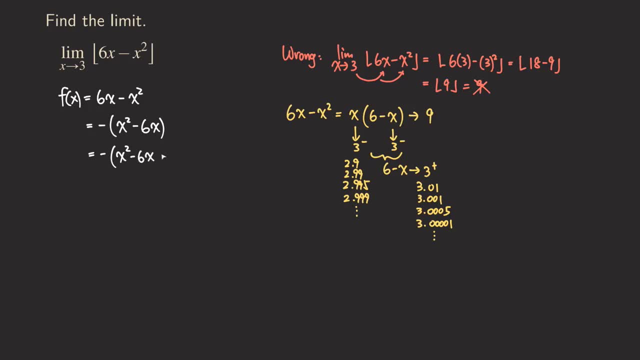 then X square minus six X, And then now, to complete the square, we need to add the square of half of this, And so what happens is that we are going to divide this by two. negative six divided by two, We are going to get negative three squared, We get 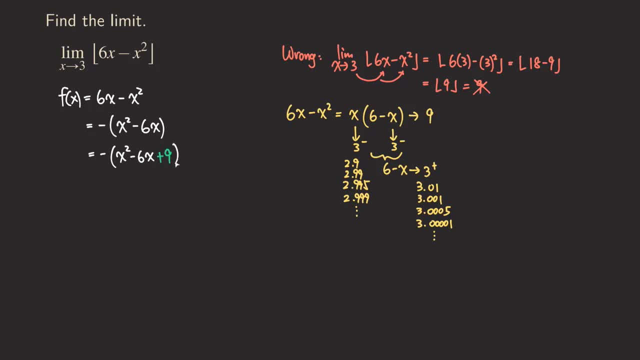 nine. So we are going to add nine here Now after adding nine, we cannot. we are changing the problem. So we cannot change the problem. So we need to do something to negate this effect. So we actually subtracting nine because, even though we're adding nine here, but because there was a 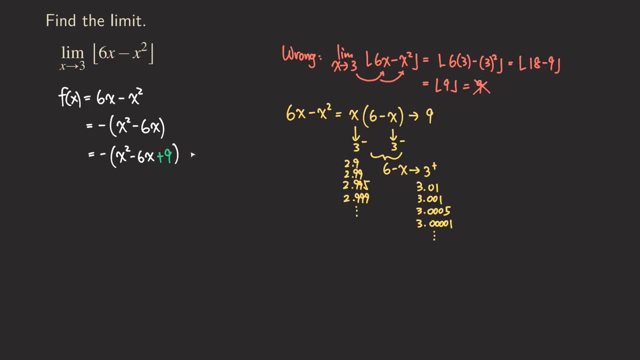 sign: here we are subtracting nine, So we actually need to do what we actually need: to add the nine back. And so that is the original expression And this: when we complete the square, we are going to get negative and then we get X minus three, square plus nine. So, rewriting this expression, we can. 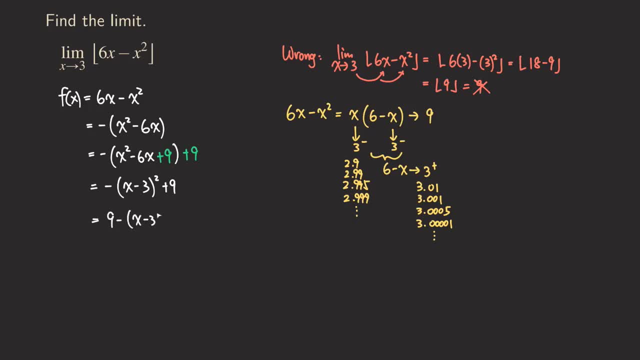 simply just write it as nine minus X minus three square. Okay, So this six X minus X square is turned into nine minus X minus three, and then quantity score. Okay, Now let's take a look at what happened. Okay, Now let's take a look at what happened. Okay, Now let's take a look at what happened. 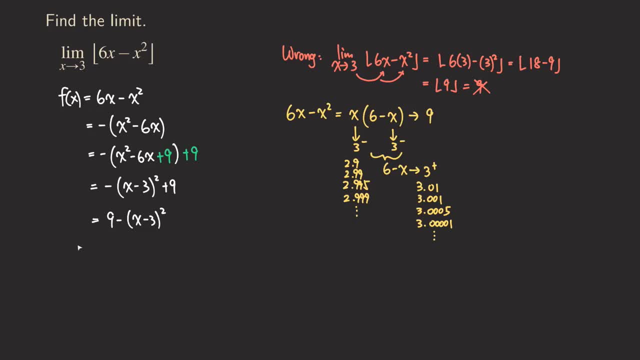 What happens when X is approaching three? So when X is approaching three, okay, what happens? Then? we can consider this: X minus three. We know that X minus three is approaching zero, either on the left side or the on the right side, but because there was a square, 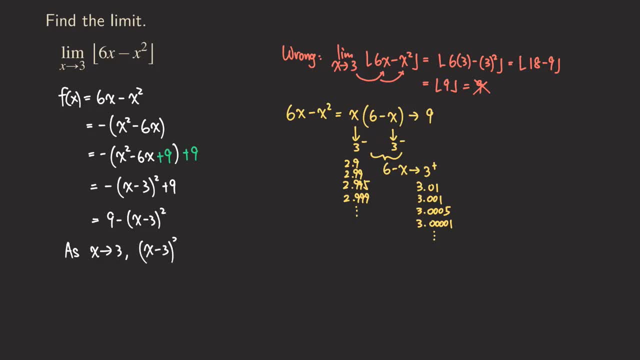 here. So we know that X minus three is approaching zero on the right side, because even if there is a negative number here, but when we square what happens, we are going to still get a positive number And this number is approaching zero. So we get X minus three, quantity square, approaching zero on. 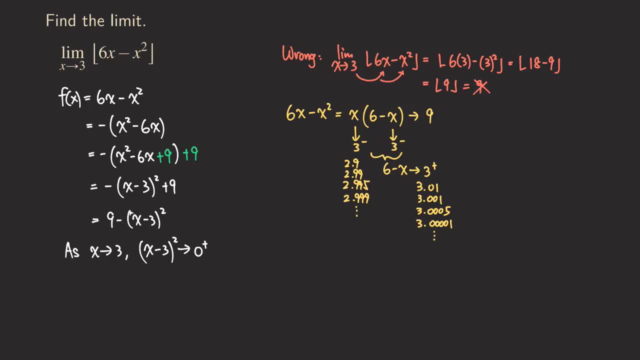 the right side. Okay Now. and what happens is that we need to consider the whole function F. right here It's actually nine minus X minus three quantity square. So because X minus three quantity square is approaching zero on the right, then we can say nine minus X minus three square. 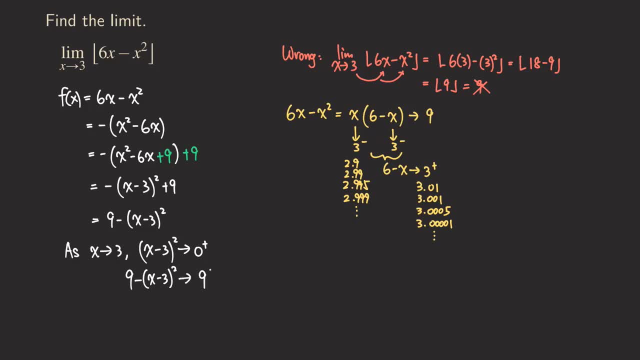 It's approaching nine Also, but it will be approaching nine on the left side. And then think about why this is true. because this is a positive number, even though it's really close to zero, but it's still a positive number. When we take nine subtracting a positive number, we are going to get a answer. 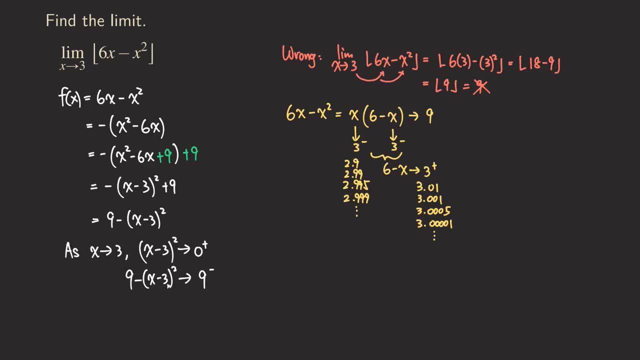 that is like eight point something. Okay, So this expression as X minus three, quantity square, is approaching zero from from the right side. this whole expression right here, this function F, will be approaching nine on the from the left side. So it will be. 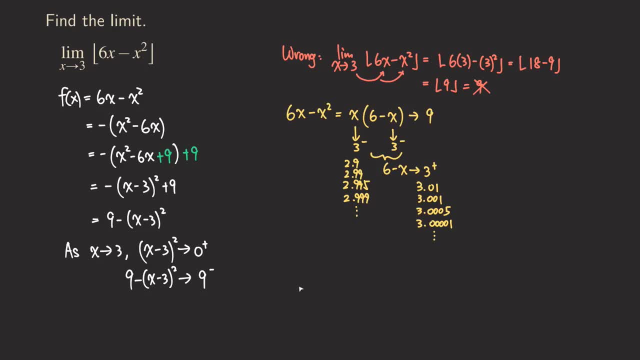 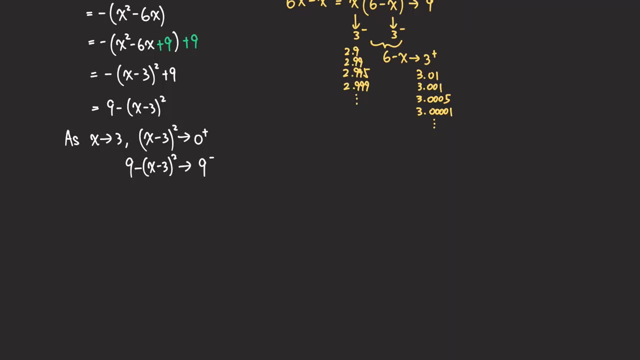 like 8.99,, 8.999,, 8.995 and so on. Okay, So what happens is that because this function is approaching nine on the left side. So now, if we consider the limit as X approaching three of six X minus X, 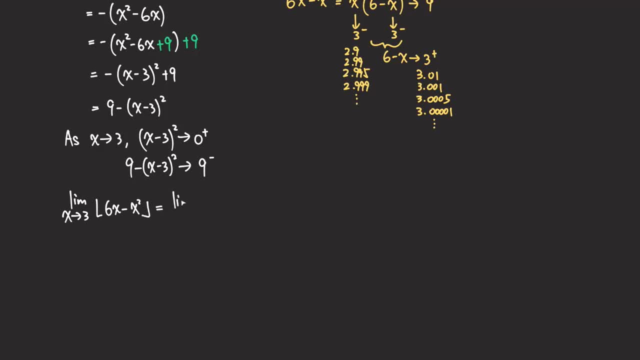 square. Okay, And then we can see that That can actually be this function right here inside the floor function. It can be replaced by the expression nine minus X minus three, quantity square, And, as you can see, this is approaching nine on the left side. And so what is the answer? Well, let's just recall something here.